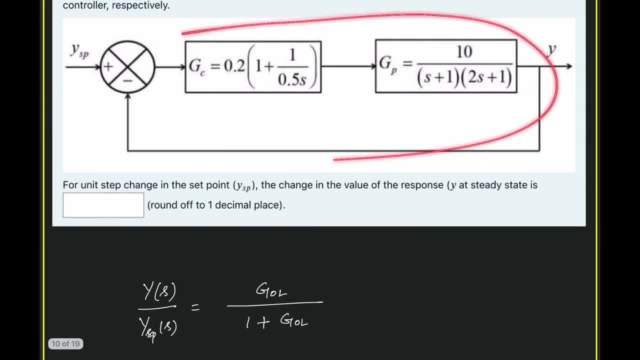 So we know, for this kind of closed loop with negative feedback, ys by ysp s is given as g o l g o l by 1 plus g o l g o l refers to transfer function in the open loop. So this open loop now is having these two components, So transfer function of this, multiplication of this, 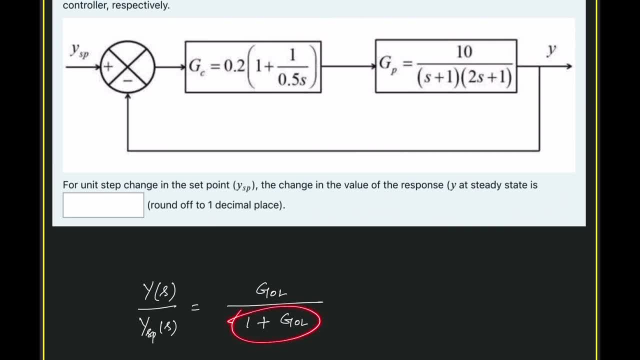 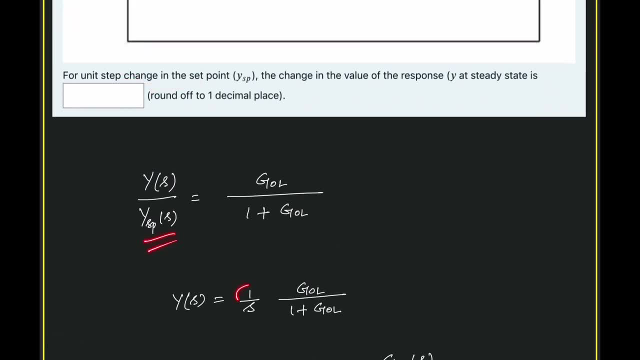 transfer function of this open loop divided by 1 plus g, o, l. okay, And we know this. ysp is for a step change in the set point, So ysp is 1 by s, ysp is 1 by s, from which ys is coming as 1 by s into. 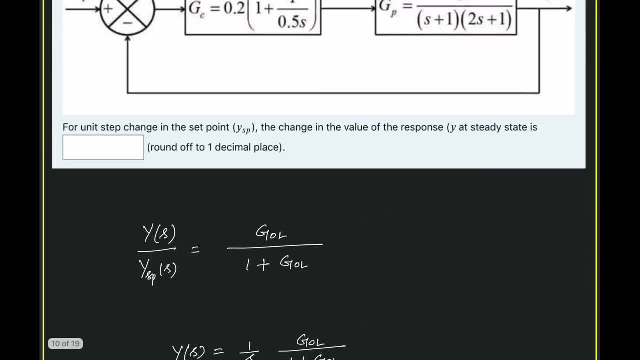 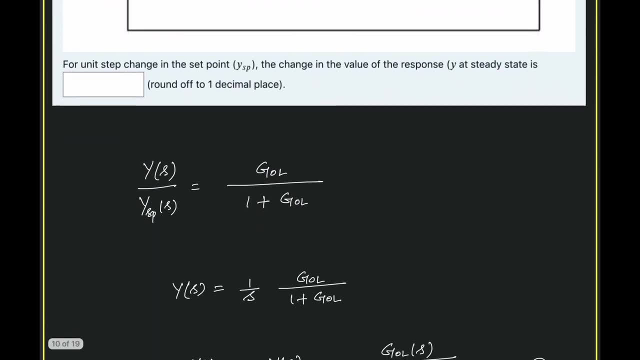 this component. So ysp is 1 by s, from which ys is coming as 1 by s into this component. And what is asked is y of t y at the steady state, otherwise nothing but the y at the final settled or the ultimate value of y conditions. So y y of t at t tending to infinity is nothing but. 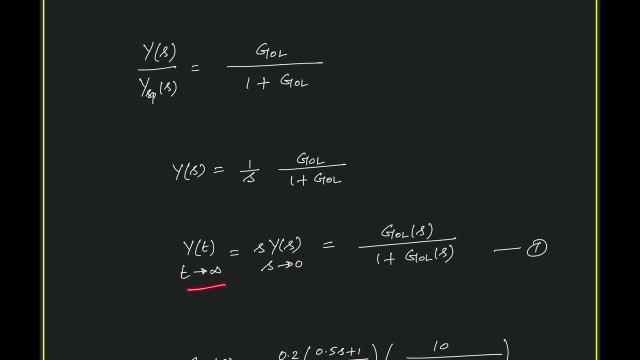 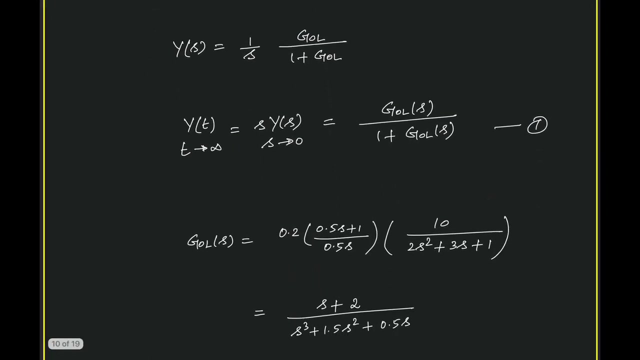 s, y of s s tending to zero. this is nothing but the final value theorem. So y of s is already this way, so s into y of s is simply equal to this into s will be getting cancelled. So we have simply again g o l by 1 plus g o l. So g o l. what is open loop transfer function? So for the open loop we have: 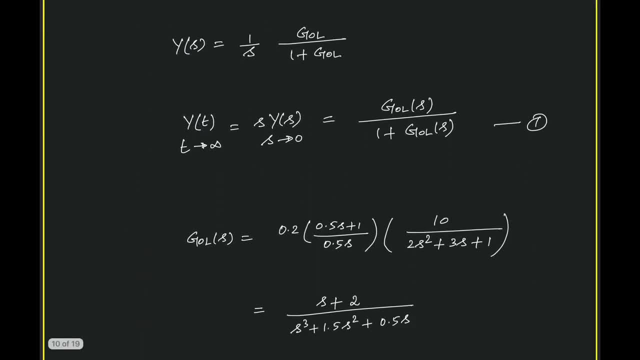 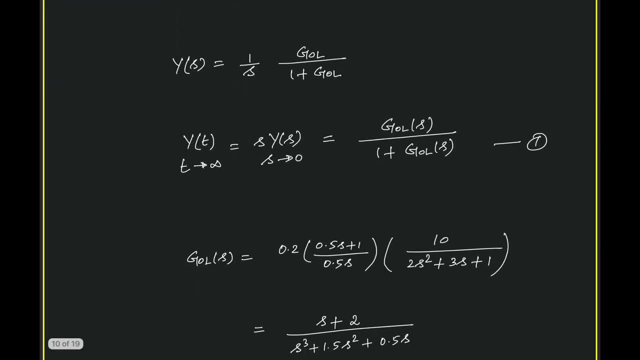 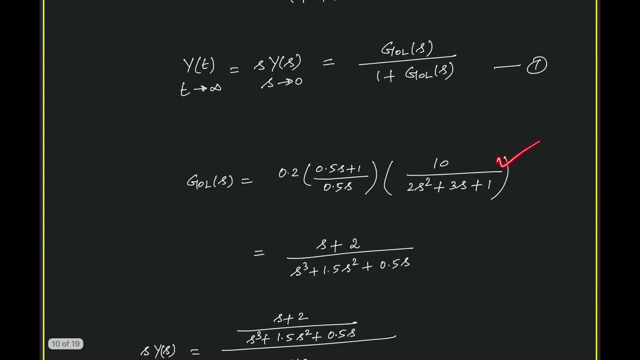 this and these two. So for that we have 0.2, or is 0.2 into this component, which is 0.5 s plus 1 by 0.5 s, And this another thing is a second order system. So we have this now available, So you can. 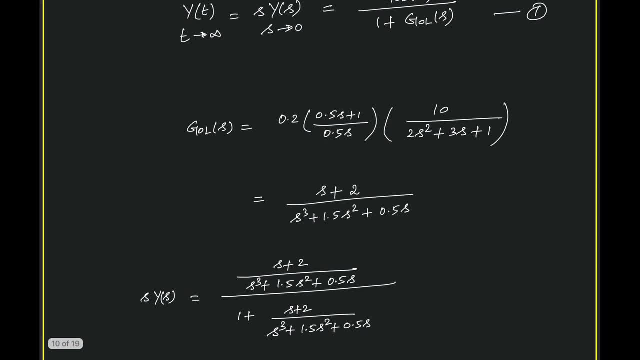 rearrange or reduce this. So this will be having 0.2, 5 into 0.5 into, so 0.2 into 0.5 into 10, which is equal to simply again 1.. So this 1 into 0.5. 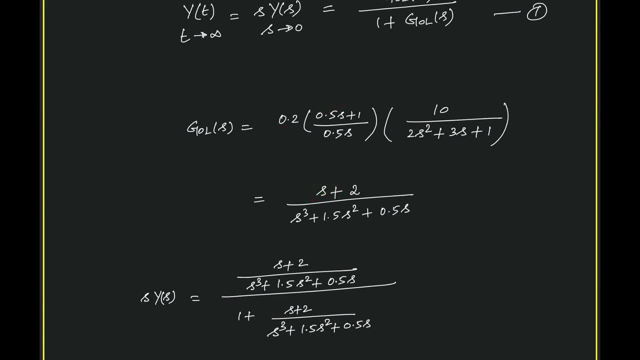 5, 5 into 0.2, 1. So we have s and 0.2 into into 10, which is equal to 2.. So this numerator is equal to s plus 2 and denominator: we have 0.5 s into 2 s square, So we have 0.5 s cube. 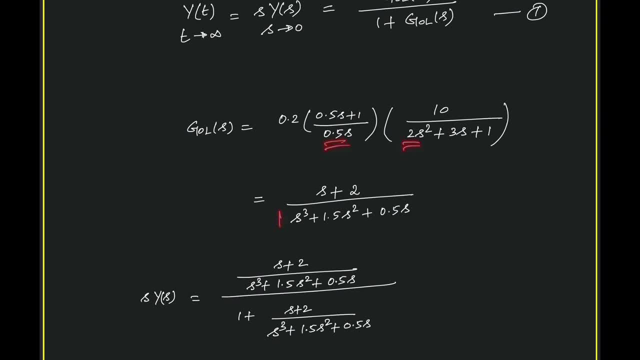 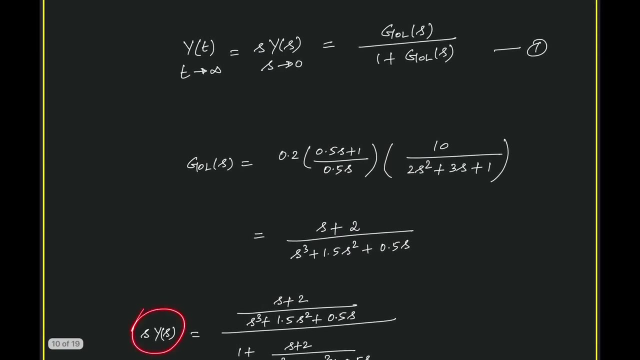 uh sorry, 0.5 into 2 now. So we have 1 s cube and 0.5 into 3 s. uh into s. So 1.5 s square, and the next last time is 0.5 s. So this is our g? o l. So what is s o s, which is nothing but g? o l. 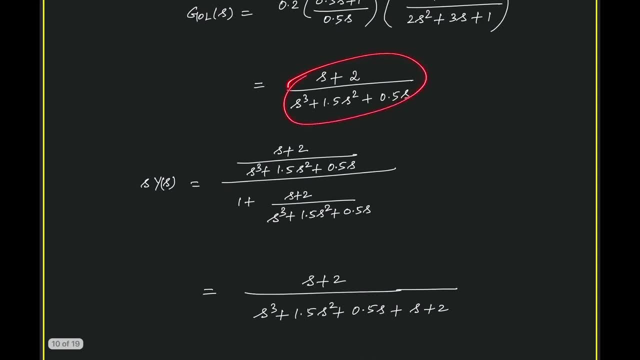 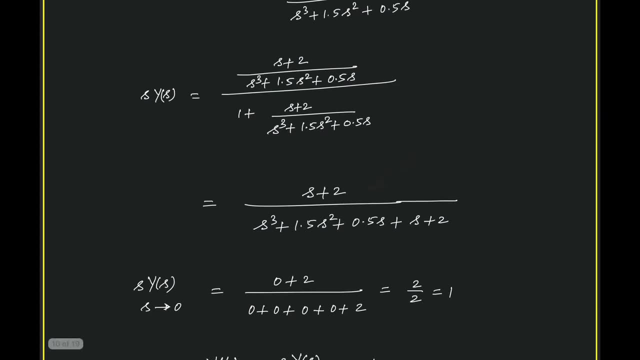 by 1 plus g o l, So g o l open loop transfer function divided by 1 plus open loop transfer function, which is 0.5 s cube plus 1.5 s square, plus 0.5 s, plus again another s plus 2.. So we can group them. 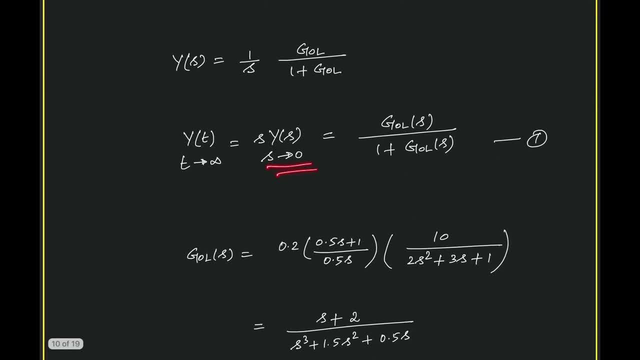 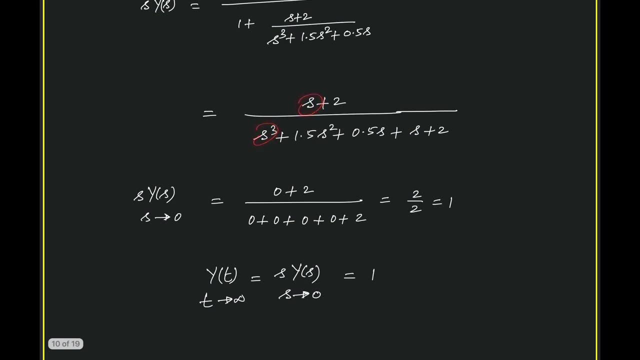 So now what is needed is s, y, s at s tending to 0, to get y of t for t tending to infinity, So substituting for s equal to 0. So everywhere we have only this numerator 2 and denominator 2.. 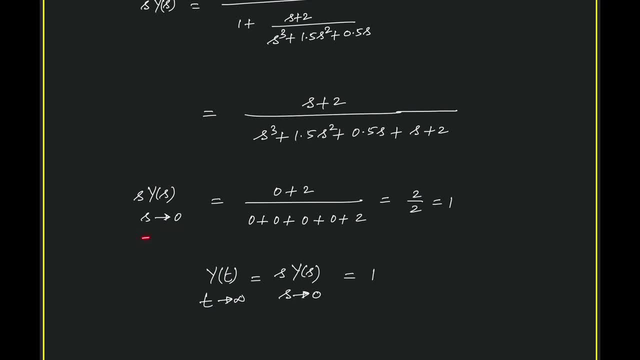 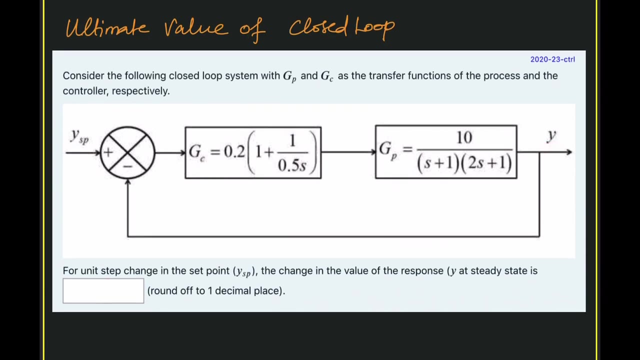 So we have s, y, s, s tending to infinite, s tending to 0, which is nothing but the y of t, uh t tending to infinity is coming as 1.. So otherwise, the final value of y is simply equal to 1.. So what it says actually, there is uh, set point is 1, output is also reaching the value of 1.. 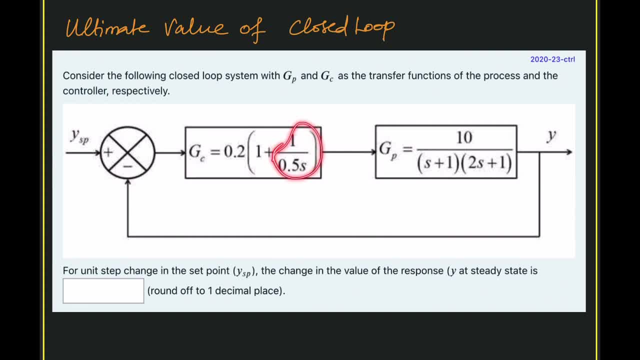 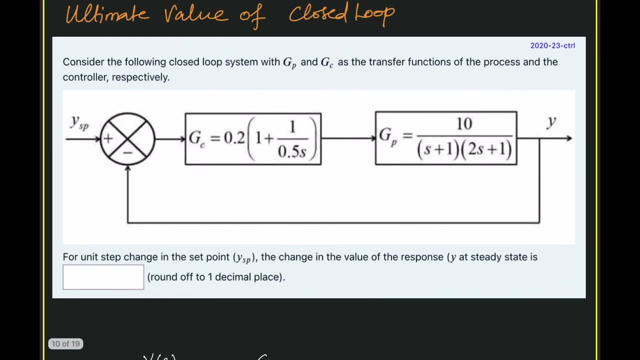 Now this is coming because of the integral action there in the controller, or is ba controller is having a integral action? uh, this is making the of offset to 0 or there is no offset. y and y sp are same, otherwise there is no offset. Additionally, we can also say about the order of the system: 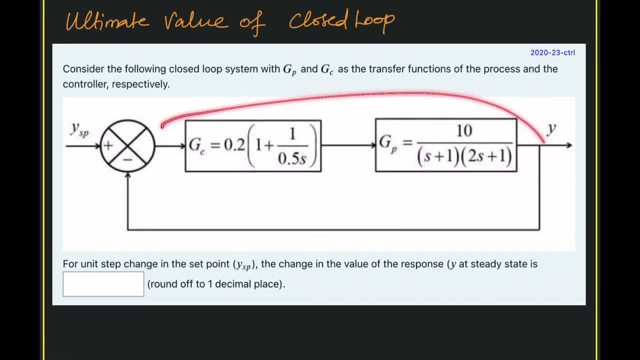 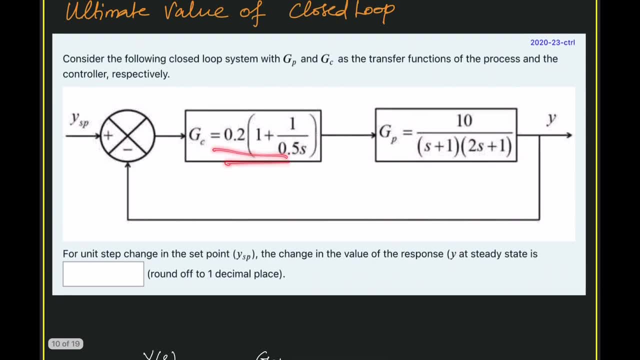 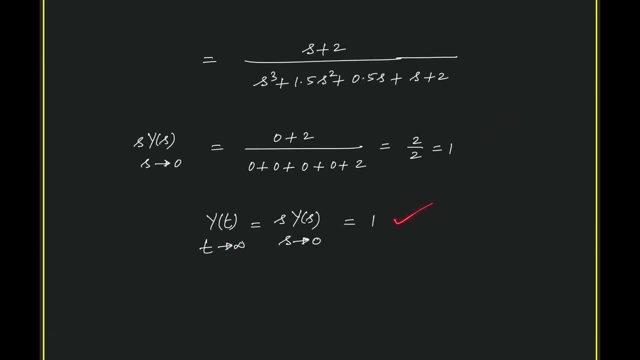 originally the system process, a second order, whereas the closed loop system is coming to be a third order. uh, because of the integral action of the ba controller. with these are the additional information, that is, we have obtained this ultimate value of the closed loop and additionally, we can: 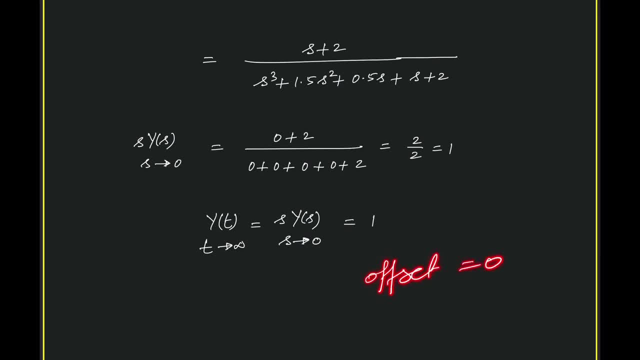 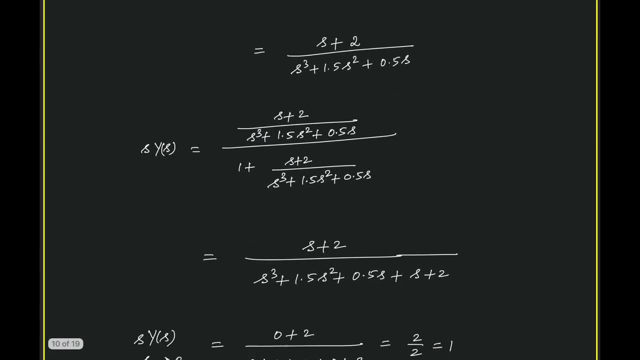 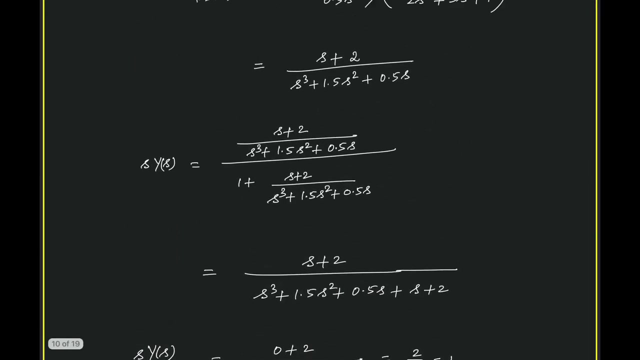 also say that offset equal to zero and the order of the system got increased. Initially it would. it is a second order system which is turning to a third order system. this is the because of the integral action service. the integral action leads to uh, eliminating the offset, but it is.